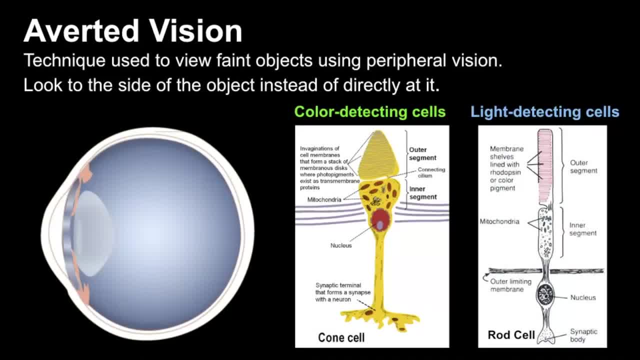 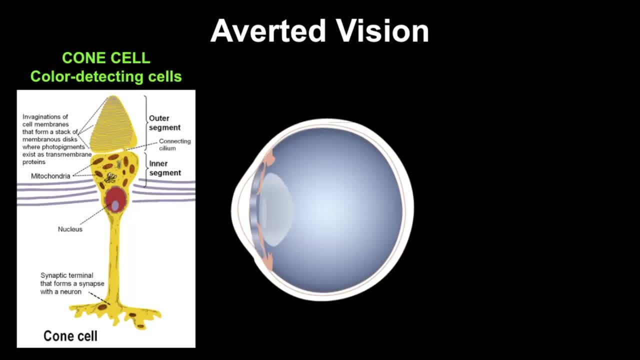 Now let's take a look at the structure of the human eye in order to understand how averted vision works. You have two types of cells inside of your eye. The first is called the cone cell, and these are your color detecting cells, and they are highly concentrated in the back center of the eye. 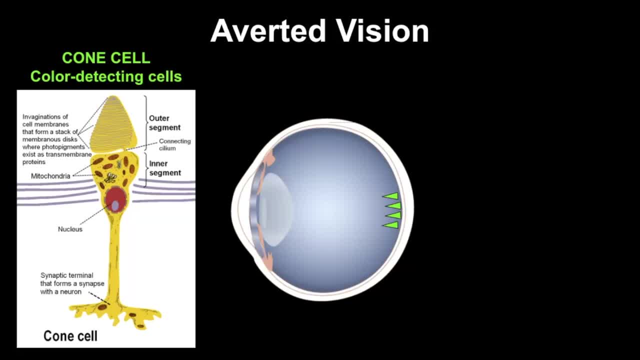 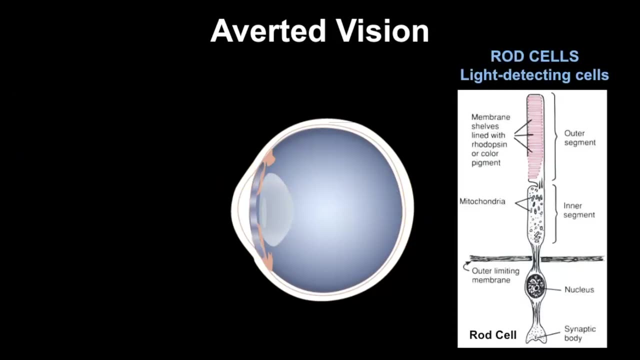 The cone cell is the center of the human retina and these cells are really responsible for that sharp, detailed vision that you can have in bright light as well as color vision, But this area of the eye is not particularly sensitive to light. In terms of light, we use rod cells and these cells 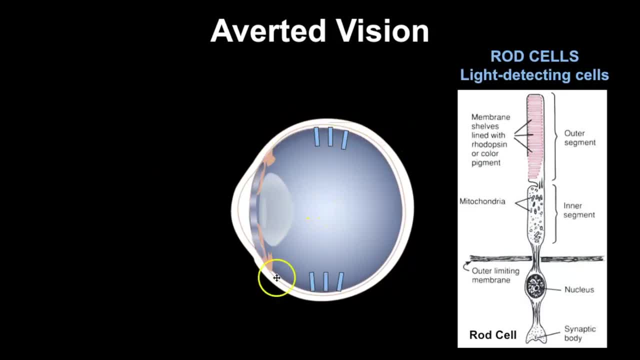 are concentrated more on the side of the eyes, right here, and these areas are very sensitive when they're in low light. So if you have a lot of light, and you have a lot of light and you have a lot of light levels, but it doesn't really allow the eye to see color. So when you're looking at an astronomical 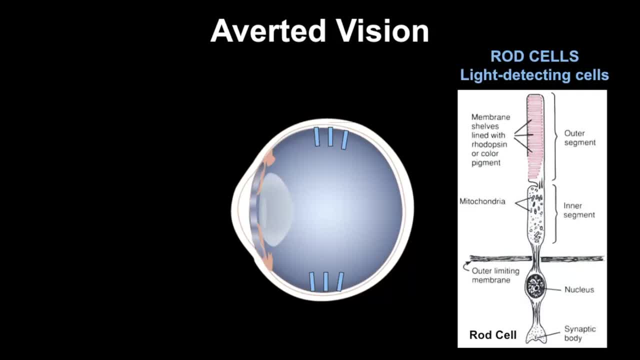 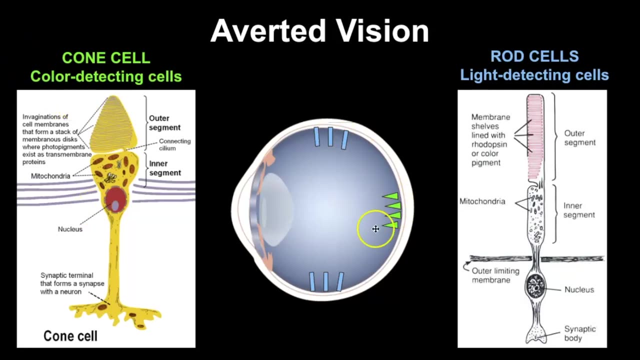 object that's far away. what you want to do is look to the side of the object. This way you're activating these cells, the rod cells that are detecting light. So, just to put this together, you have two different types of cells. You have cone cells that are concentrated in the center. 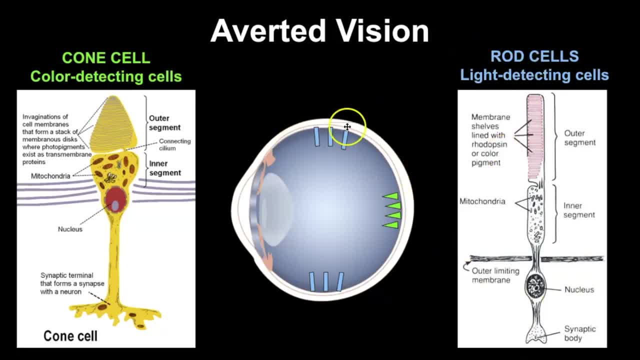 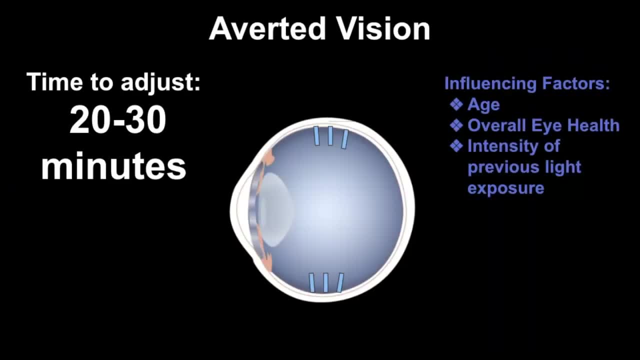 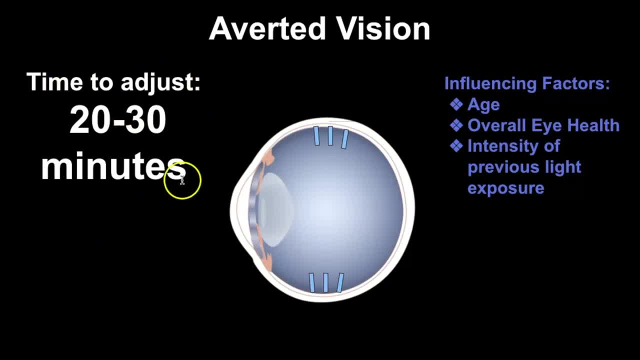 changes over time, And then what you're going to do is look to the side of the eye. It is important to note that averted vision only works when you give your eyes enough time to adjust. Typically, it takes between 20 to 30 minutes for your eyes to adjust through a process called. 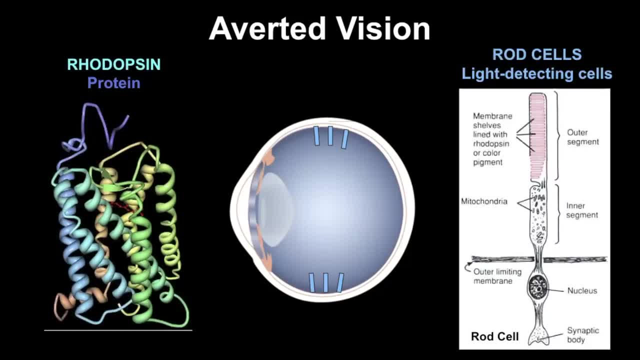 dark adaptation. There are some factors that influence this, such as age, overall eye health and the intensity of previous light exposure, and it's a light-sensitive protein that's found in the rod cells of the retina in the human eye as well as many other animals, And when a photon of light strikes the rod cells. 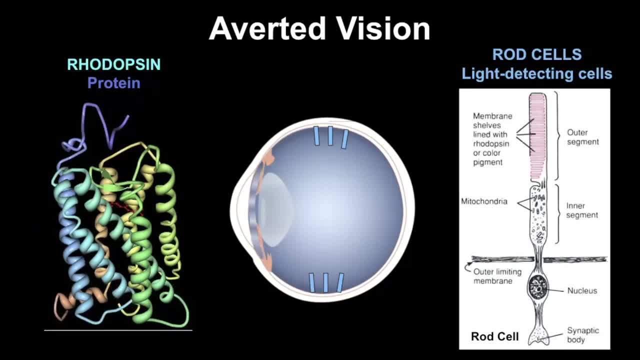 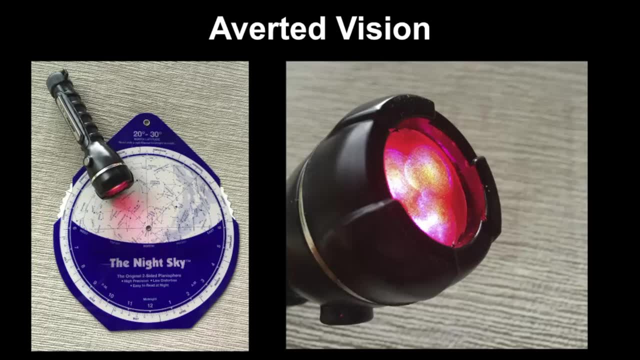 the rhodopsin becomes activated and allows the eye to perceive objects in low light conditions. Another thing that's important to acknowledge with averted vision is making sure you maintain your night vision. So using red light is very important because it has the least effect on dark. 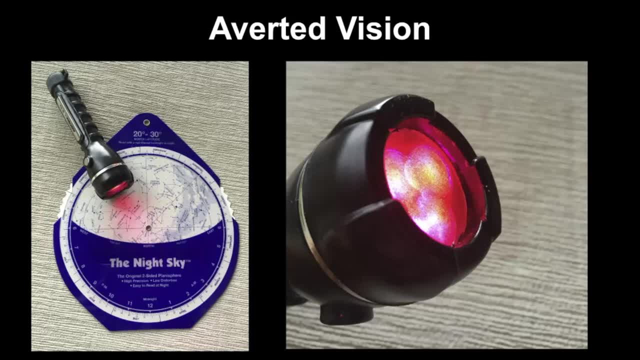 adaptation. The human eye is less sensitive to red wavelengths, So using red light is something that's very common when you go out to stargazing star parties. And here what I do for my red light is: I usually find a flashlight that I may already have and I paint it with red nail polish. So 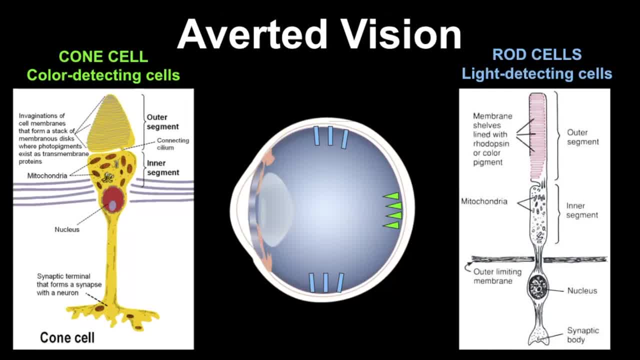 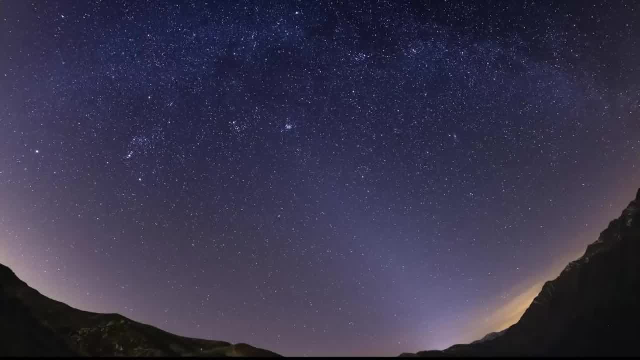 again, averted vision is something that takes a little bit of time, but it's a very important time, and practice patience, but you also need the right conditions To use averted vision. astronomers deliberately look to the side of an object they want to observe By doing this. 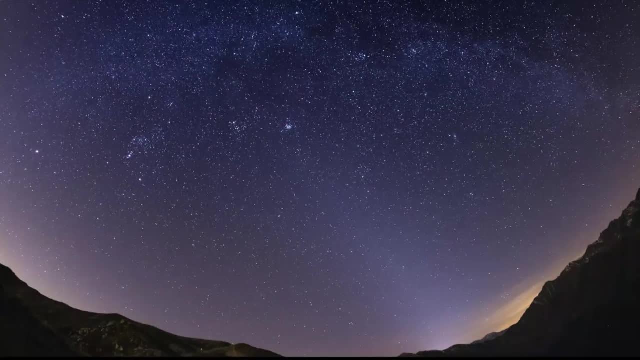 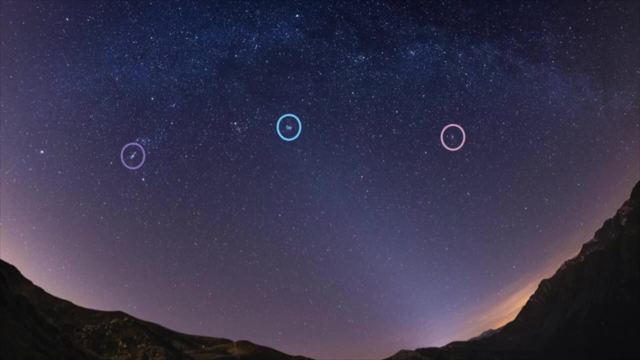 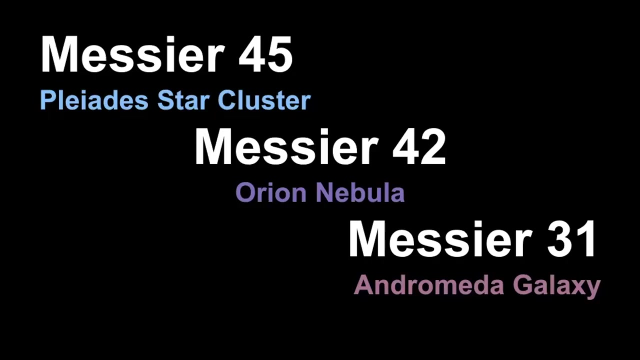 the faint light from the object is hitting the more light-sensitive rods that are on the side of the retina. So which objects could you look at? in order to practice this technique? I came up with three objects that you can focus on: on The Pleiades star cluster, Orion's nebula and the Andromeda galaxy, All three of which are in 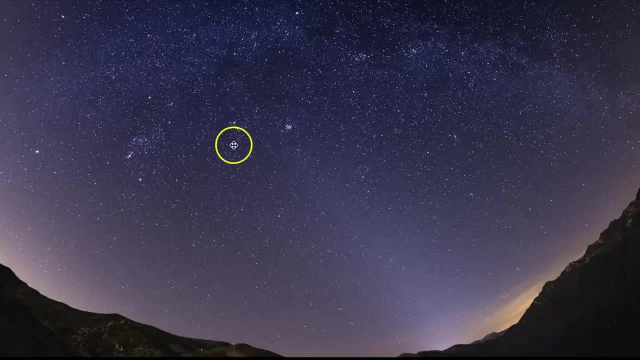 this photo that is pictured right here. So first my eye is drawn right here that's the Pleiades, and I have a whole video that goes in depth about this star cluster. so if you want to learn more, go see that video. But here is the Pleiades, right here is Orion's nebula and then the Andromeda. 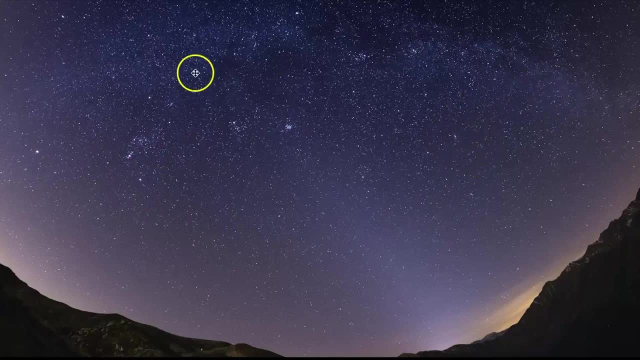 galaxy is right here And this is a great photo because you can see all of those and actually you can see zodiacal light coming off kind of in this cone shape off the horizon here, And I do have a video about what zodiacal light is, so go see that if you want to learn more. So the Pleiades. 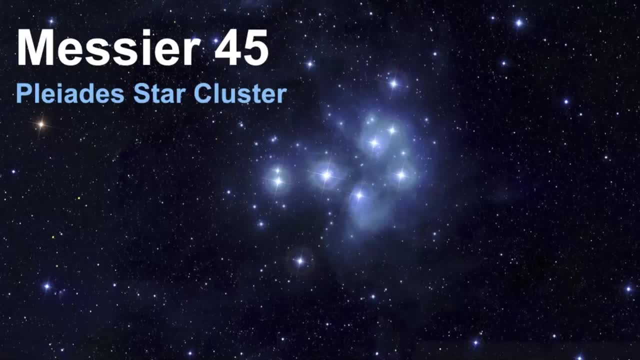 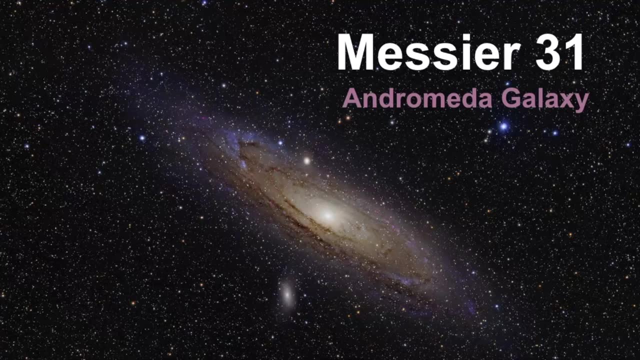 star cluster. that's an object you can focus on Messier 42, which is Orion's nebula, and Messier 31, which is Andromeda's galaxy. Let's get a little bit more practice looking at some photos so you can start to learn how I identify these objects. 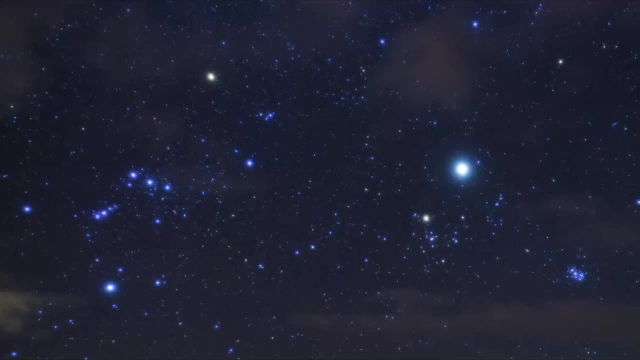 So there are two objects that I mentioned: the Pleiades, which is all the way to the right side, towards the bottom of the photo, and then you have Orion's nebula, which is more towards the left side. here is where the Pleiades are. To me, that's the most recognizable star cluster. to most people. 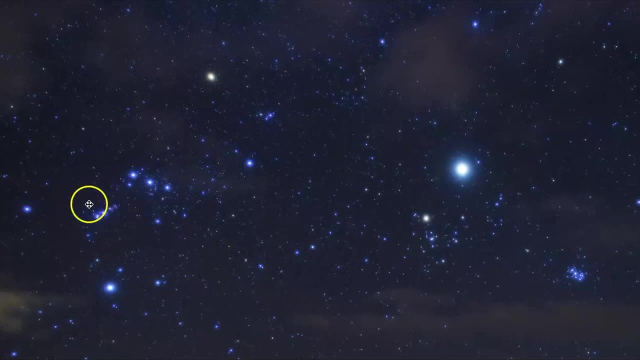 and then over in this region is where Orion's nebula is. now it doesn't really show up as well as, say, Titan or Mercury, actually, when we get closer. but in this plus circle, here is where Orion's nebula is Now it doesn't really show up as well as say, Orion's nebula is straight in the circle center. This is앙 the Typosic from Nebulaups, of Orion's nebula nebula and then over in this region is where Orion's nebula is. Now it doesn't really show up as well as. 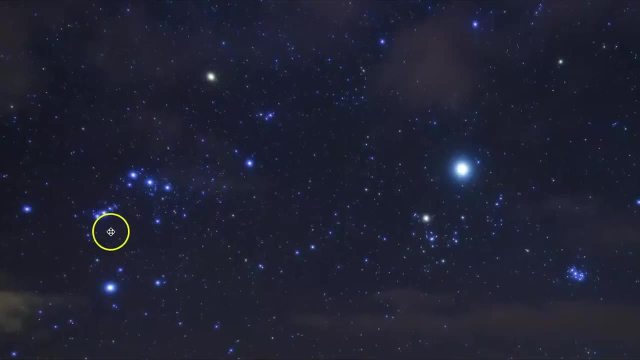 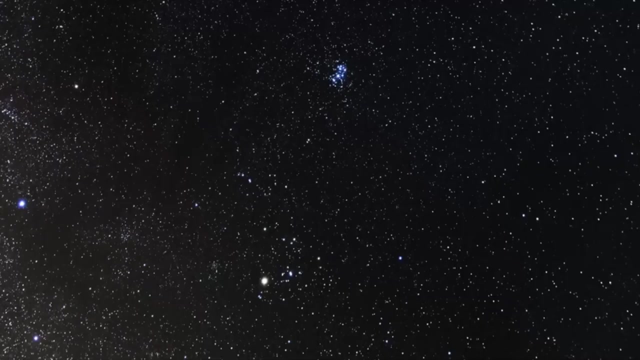 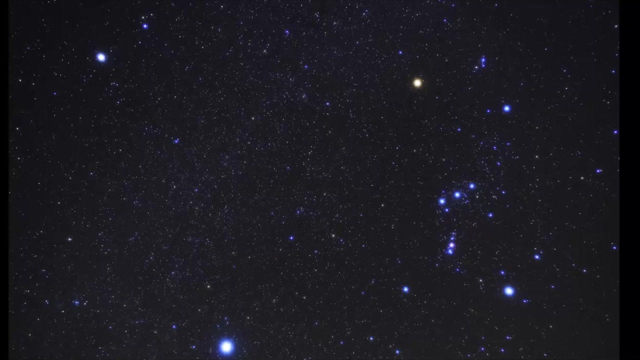 this photo, but it does give you an idea of where it is, and it's right beneath the belt stars. Let's get another practice photo. Here we have Taurus, and hopefully your eye is drawn to the Pleiades star cluster right here. And here's another photo. Here we have Orion, towards the right side. 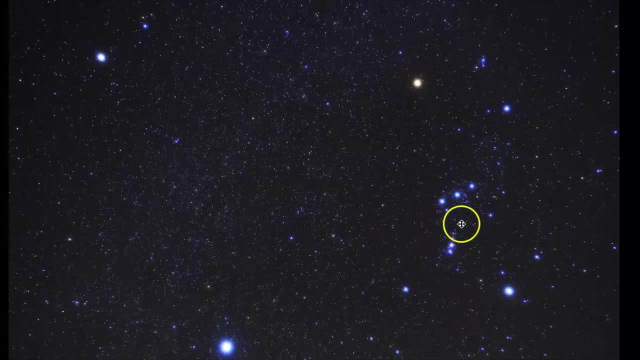 Here's Orion, Here are the belt stars, and Orion's nebula is right here. So when you're looking at this object in the night sky, you want to look to the side of the object and then again that light is going to hit the side of your eye that is able to detect light in low level conditions. The 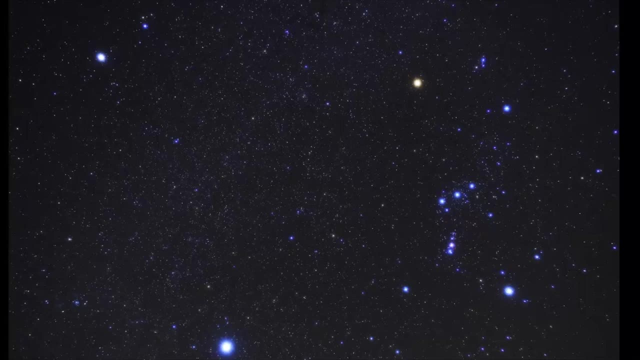 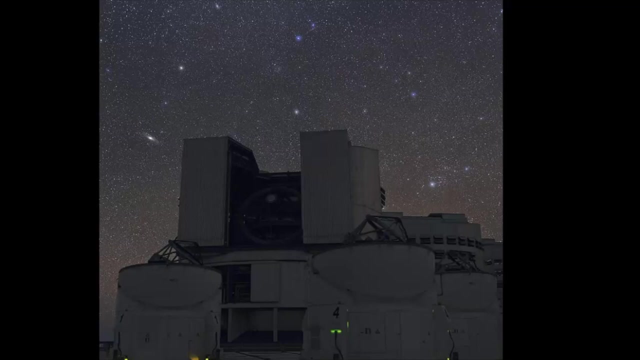 trade-off is you. you kind of lose that sharp focus. but again, just a technique for you to practice. I've got one more photo here. So here: I love this photo because it shows you Andromeda in the background, and this is Andromeda galaxy. 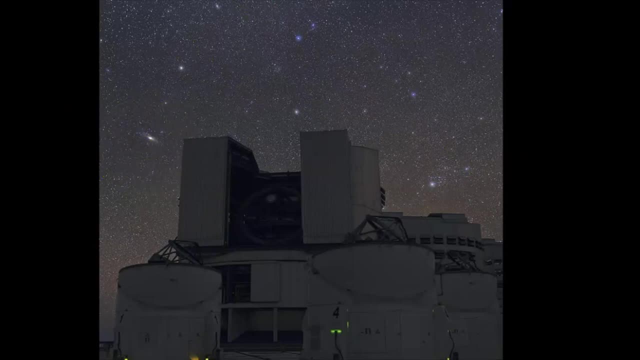 So when I go outside to see this, this celestial object, you really need dark skies and it's helpful just to look to the side of the object, not directly at it, and what you see is it'll start to come into focus a little bit more because you're activating those rod cells. 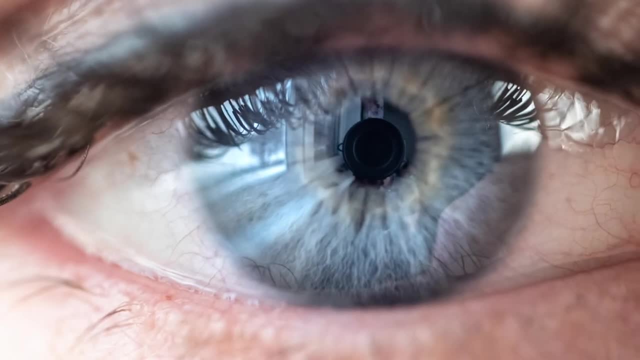 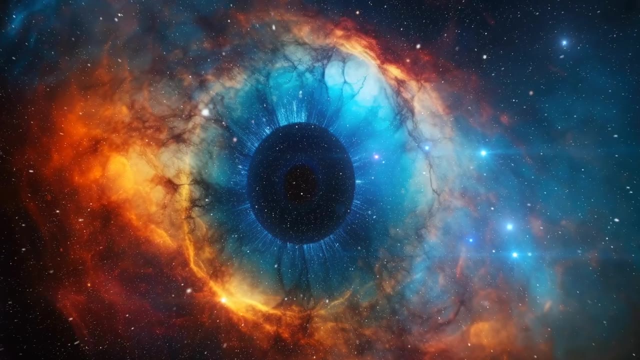 As I was making this video and talking about the structure of the human eye, I was reminded that there are objects in space that really look like human eyes, And I know I'm not alone. They're the one that has the most fascinating actual eye or lumen eye. But what I want to cover with these eye, 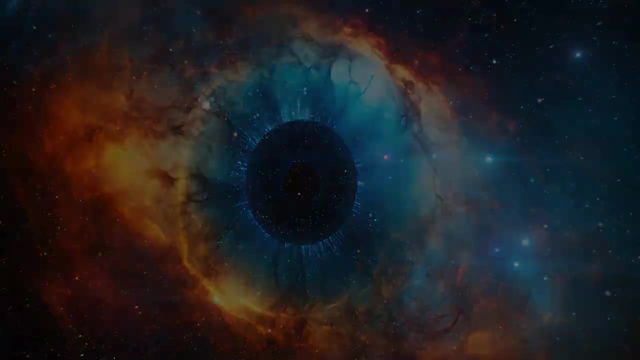 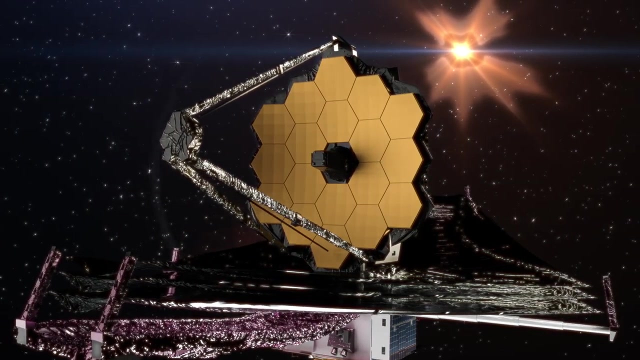 eye point hills, which I really wanted to focus back on today. is this depicted here? There were a lot of in thinking this. Our human eyes are very limited So as I was making this video, I just felt very thankful for those artificial eyes that are out there that are able to see the things that human 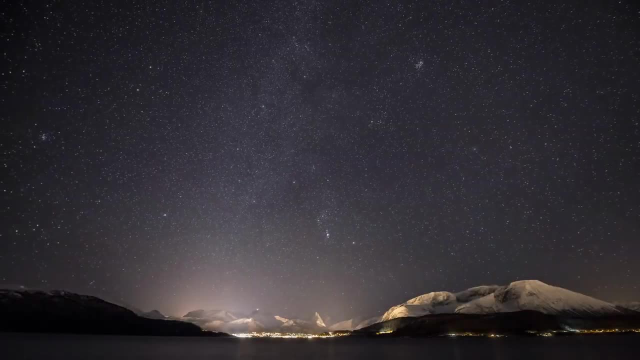 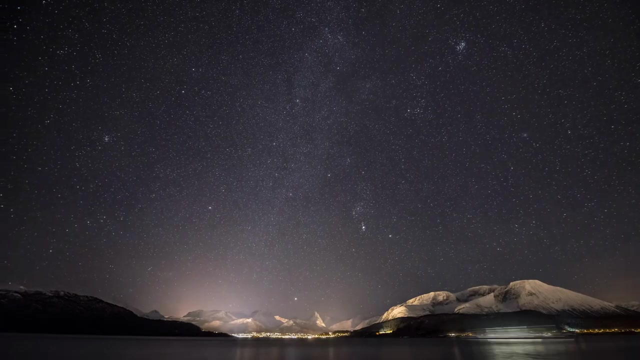 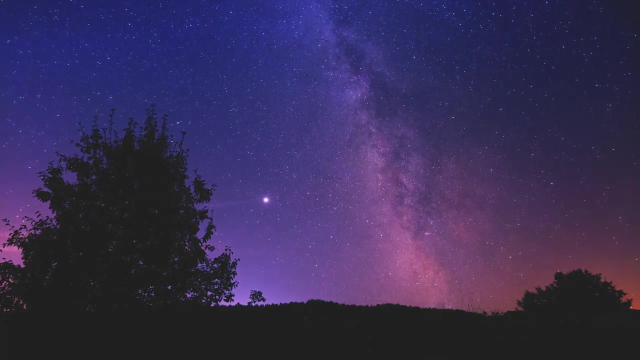 eyes cannot. So let me know in the comments below: have you used this averted vision stargazing technique And, if so, which objects have you practiced with in the night sky? Remember, it takes time, patience and practice to stargaze. So take a friend with you. give your eyes time to.